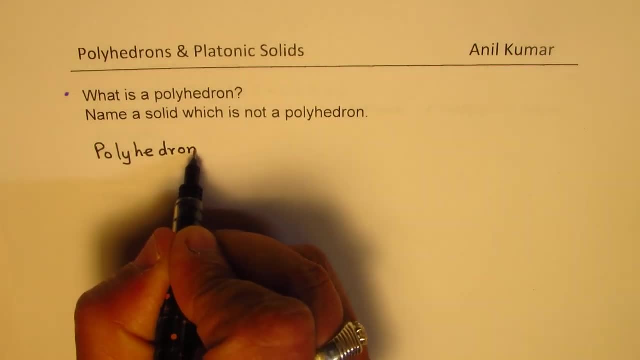 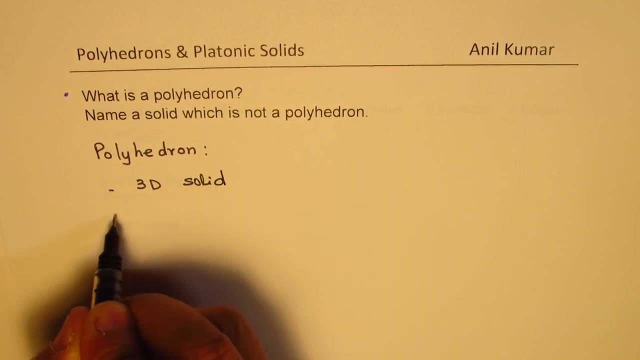 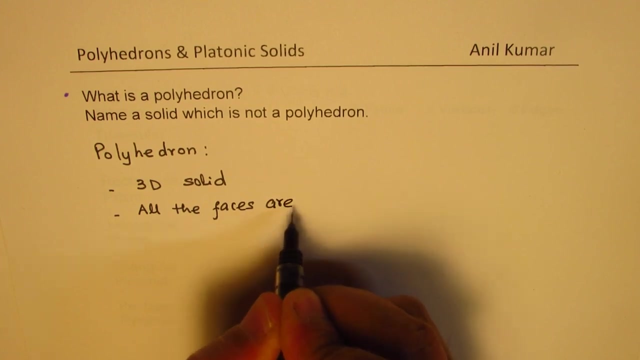 So it has a 3D shape. So it has few properties. First, it is a 3D, solid right. Second important property which it has is that all the faces are polygons. All the faces are polygons. Okay, Now it is important to note here that there could be different kinds of polygons. 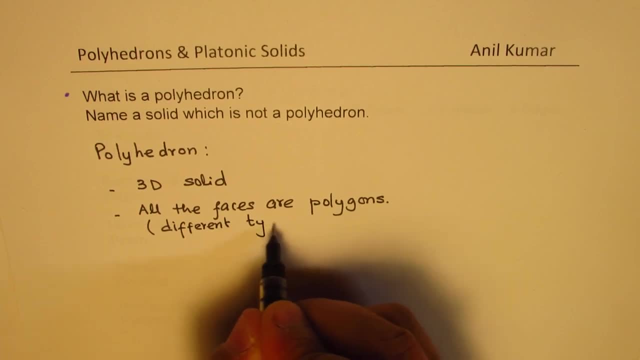 or could be different types of polygons, right, But all should be polygons. That is kind of very important right Now. then the important thing here is that these faces, they intersect in a line which is called an edge right. so so in a polyhedron we have edges. 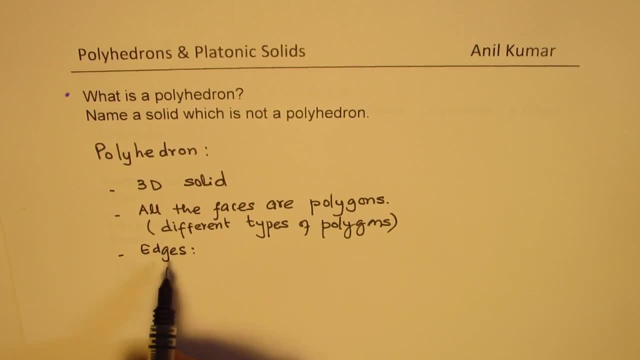 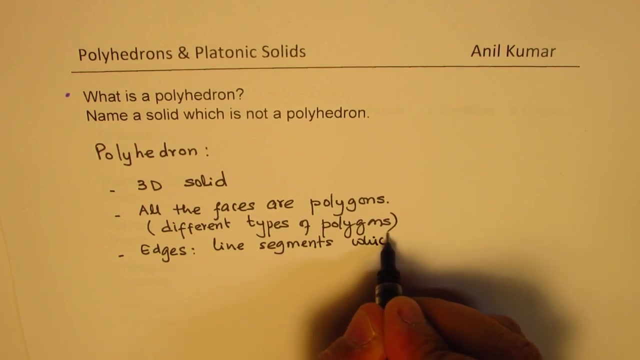 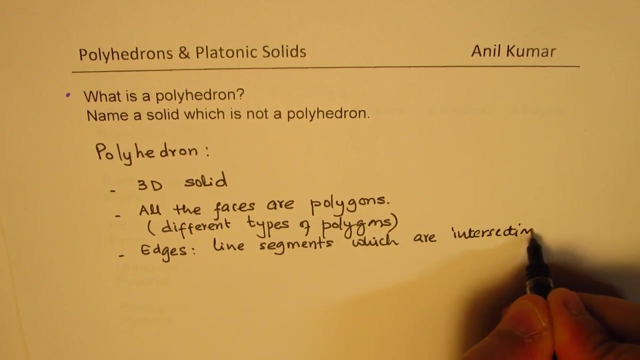 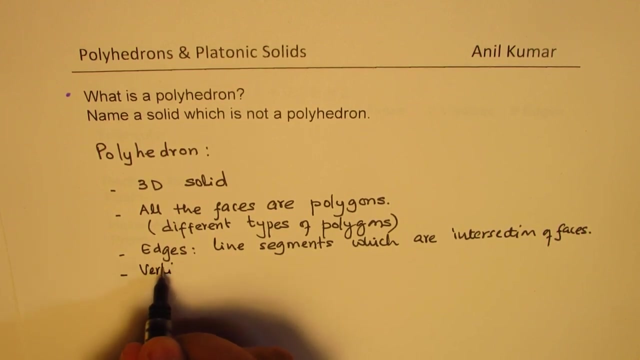 and these edges are basically line segments. intersection of faces. so the faces of a polyhedron will always intersecting to edges right and the edges will meet at vertices. so we have vertices also. so as far as what is, is are concerned, we it are the points where the faces intersect right, or you can say that the edges. 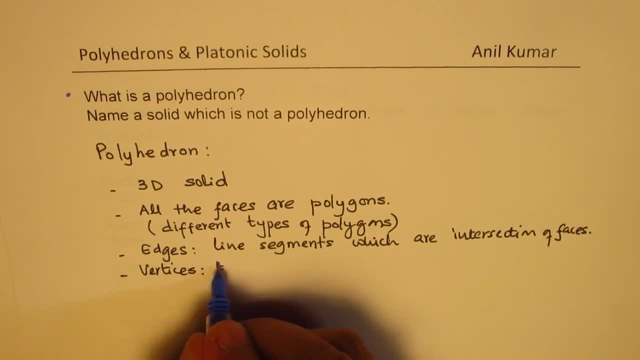 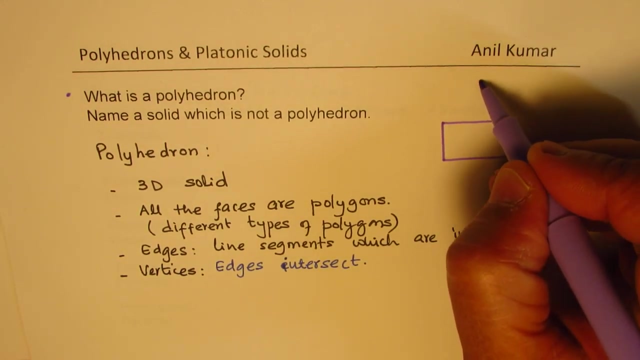 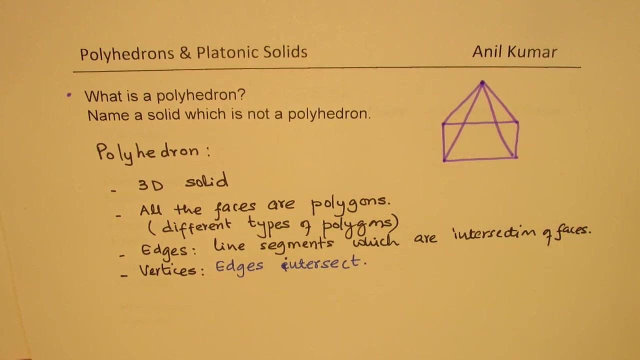 intersect, right? so we can call: vertices are where the edges intersect. so, to give you an example, let's take a rectangular shape, right now. this is rectangle, is a polygon, right? so if we have a vertex here and we can join this with different vertices, we get a shape here. Now this particular shape is a 3D, where we have one face, which is: 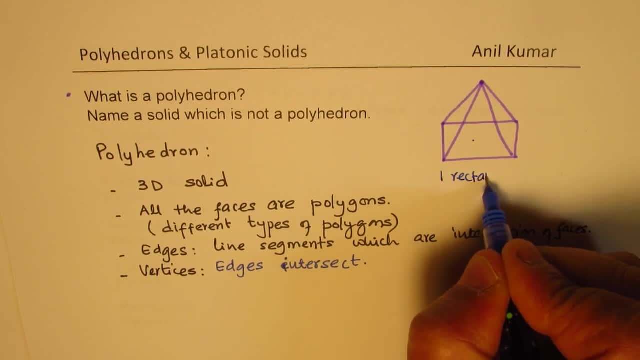 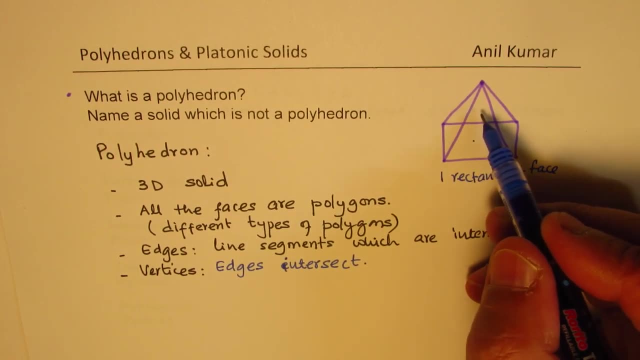 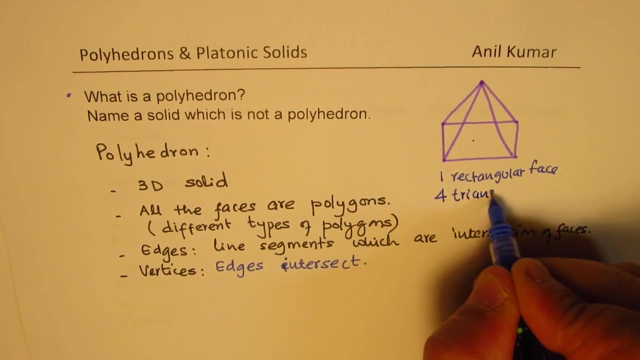 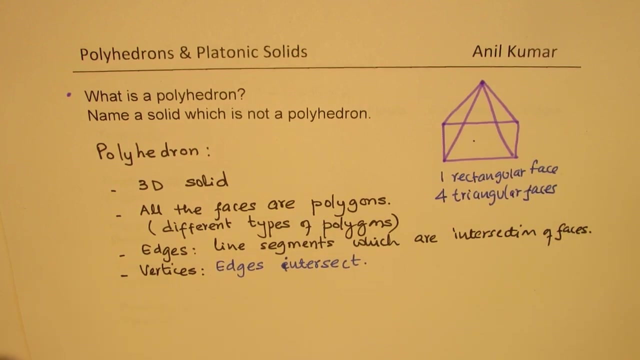 rectangular right. We have one rectangular face and we have one, two, three, four. With all those four sides and this vertex, we have four triangular faces. Now, that is a polyhedron, because all the faces are polygons, correct? That is a polyhedron. 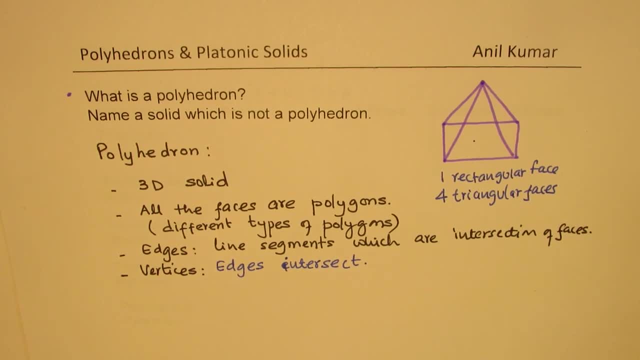 Now these faces are polyhedron. because they are polyhedron, Now these faces, they intersect. So you see these faces, these are the faces. Let me shade the faces first. What we are saying. this is a face, right Base, This is also a face. These are the faces. 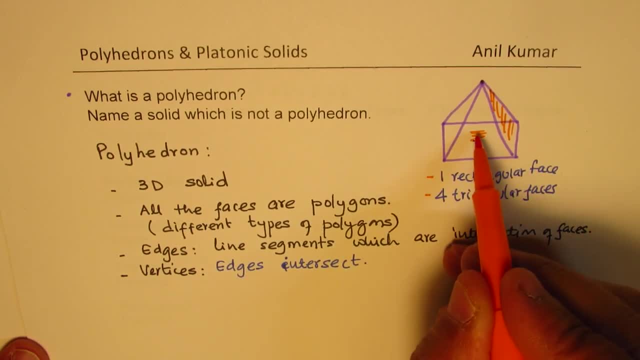 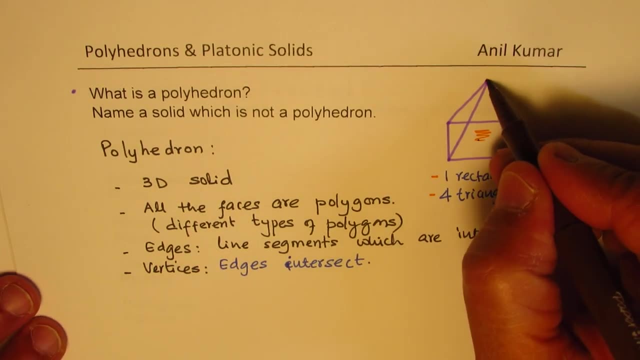 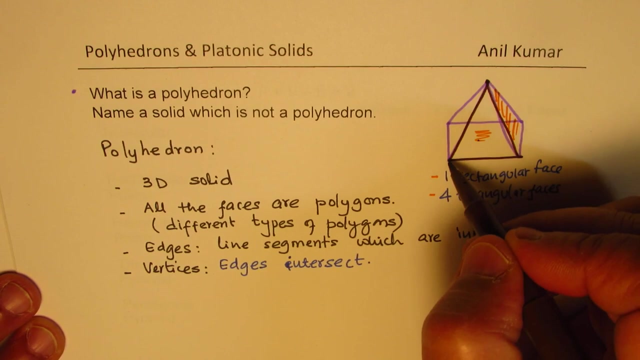 which we have mentioned as one rectangular face, which is the base, and four triangular faces. And these are the edges. What do you see? These are the edges. So this edge is because of these two faces intersecting. Do you see that? So we have how many edges? We have four at the bottom and four going to the vertex. We have 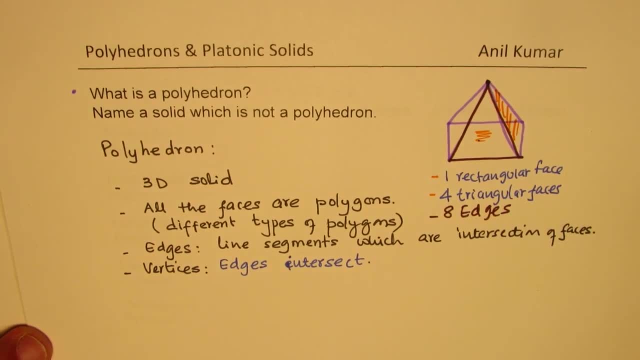 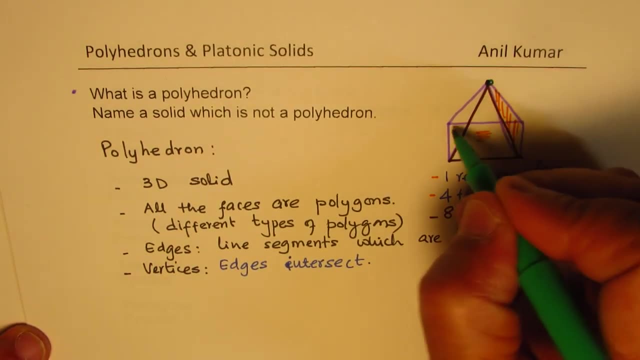 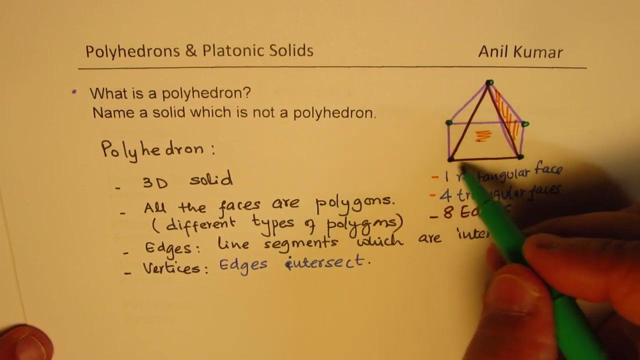 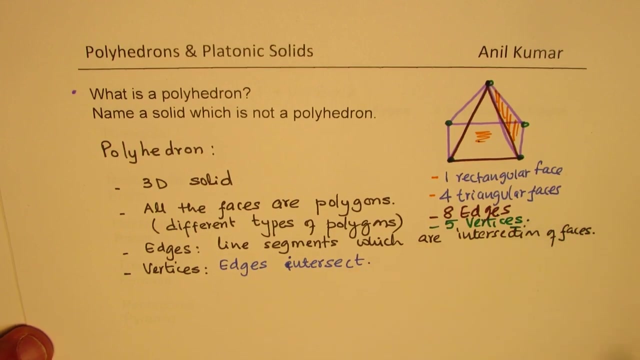 eight edges. Is that clear? Now these edges, they intersect at some points, and these points are the vertices, Correct? So one, two, three, four and one five. So that is how we have a well-defined polyhedron. Now, name of the polyhedron is also based on. 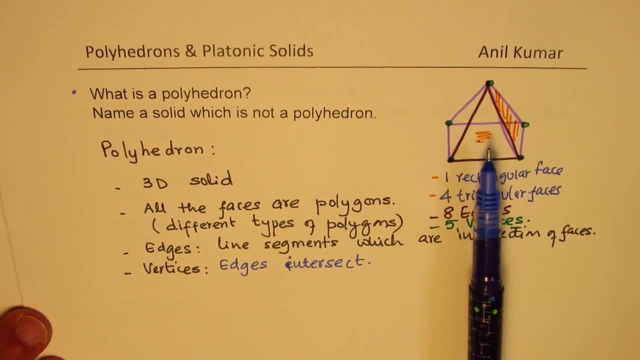 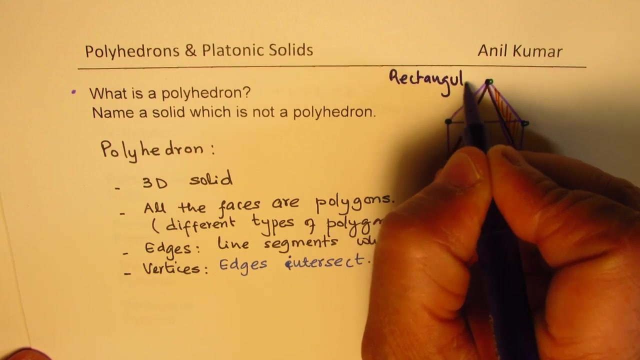 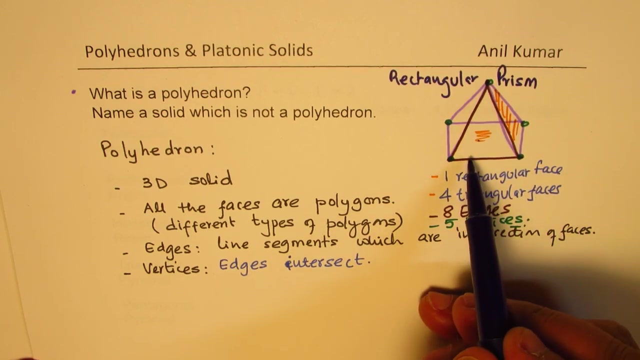 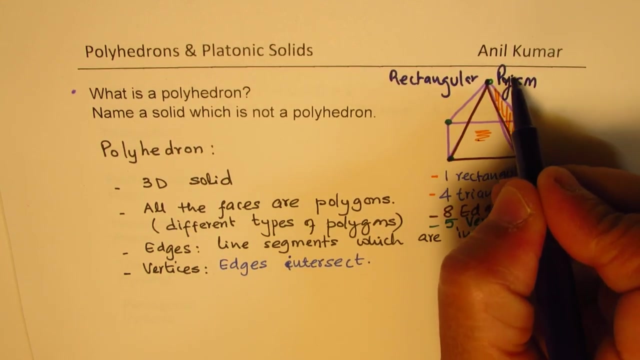 the face right. So since it is a rectangular and where everything meets at one point like this, it is a prism, So we'll name this as rectangular prism. So the name of this will be: if the other side is congruent to the base, In that case, oh sorry, pyramid, Sorry. 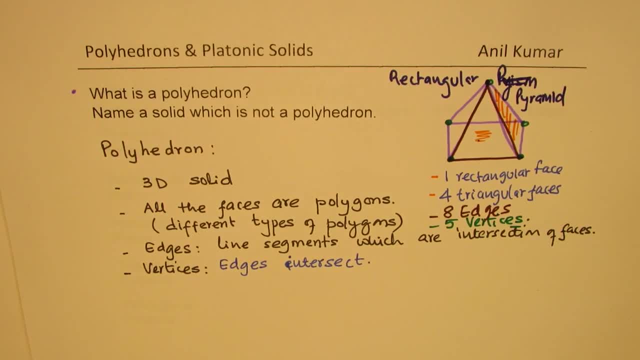 So this is a rectangular pyramid where we have one vertex on the top prism will be one in which will have the same top as the base. Okay, so anyway, this gives you some idea about what a polyhedron is. Now, the second question over here is: 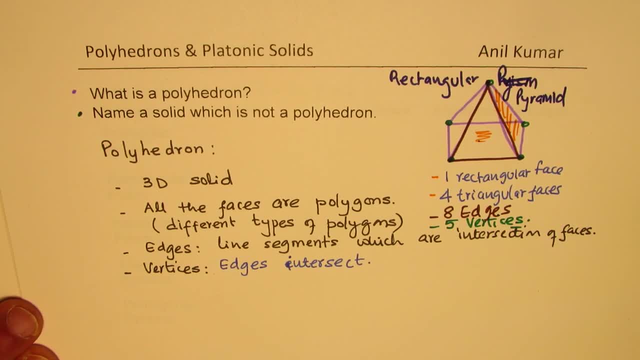 name a solid which is not a polyhedron. a polyhedron could be cylinder or even cone. Now, these solids, as you can see, this is a cone right, and then we have a cylinder which I should draw. first, The faces of cylinders. 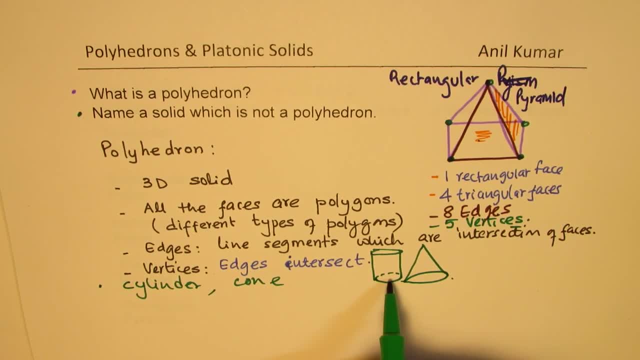 and cones are not polygons. You have this circle here, correct? and the curved surface. These are not polygons, right? So the face circle is not a polygon. So the face, which is circle, is not a polygon and therefore this is not a polyhedron. Is that clear to you? 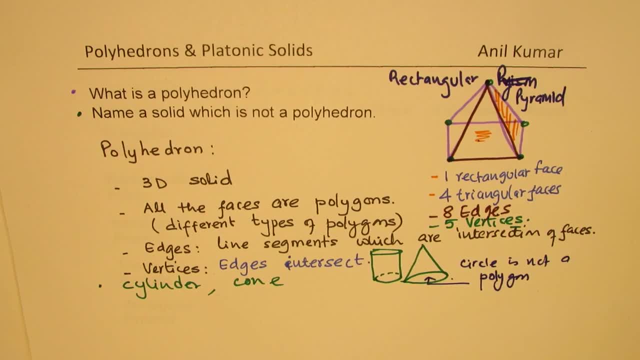 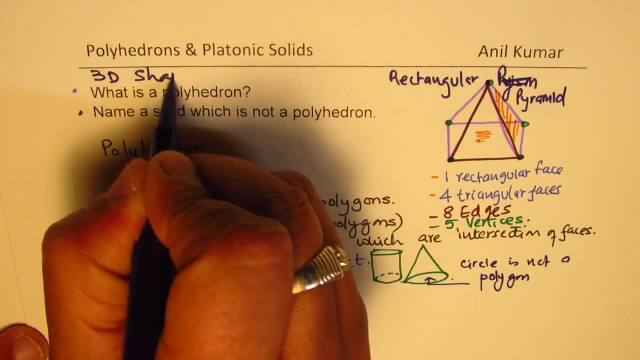 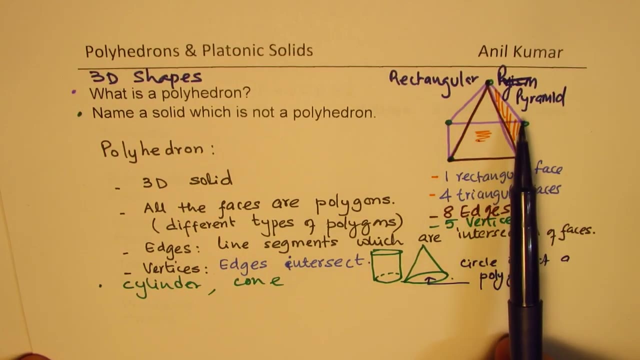 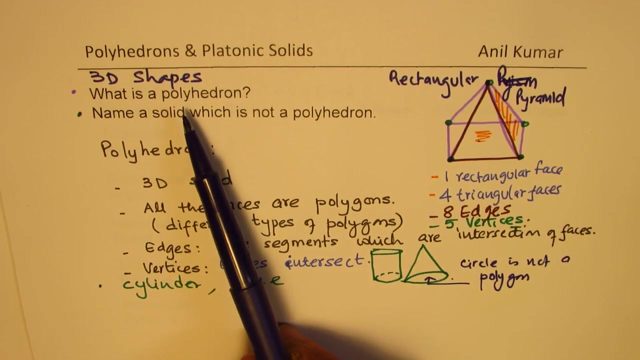 So that is how we actually distinguish between these different 3D shapes, right? So we are talking about 3D shapes here. So in 3D shapes, the ones which have polygons as its faces will be called polyhedrons. and if even one of the faces is not a polygon, in that case it is not a polyhedron. perfect. 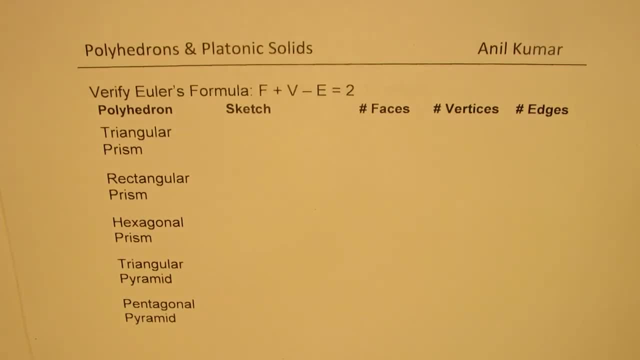 Now let's move on and talk about something very interesting, which is: we talked about what are faces, What are polyhedrons, What are polyhedrons, What are polyhedrons, What are vertices and what are edges. There is a very good formula, Euler's formula, which 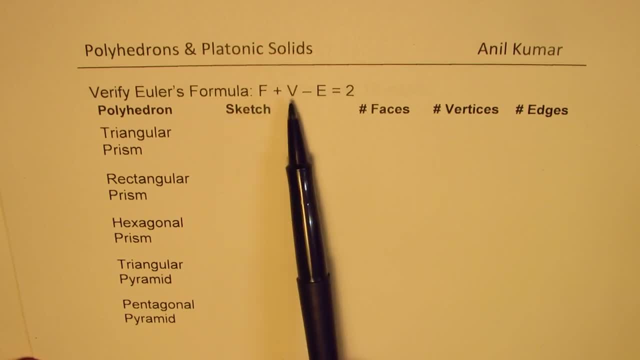 relates these numbers: Number of faces, number of vertices and number of edges. So when you add number of faces and vertices and take away the edges, you always get a number 2 for a polyhedron. okay, So let's try to figure this out for the examples which I have taken. 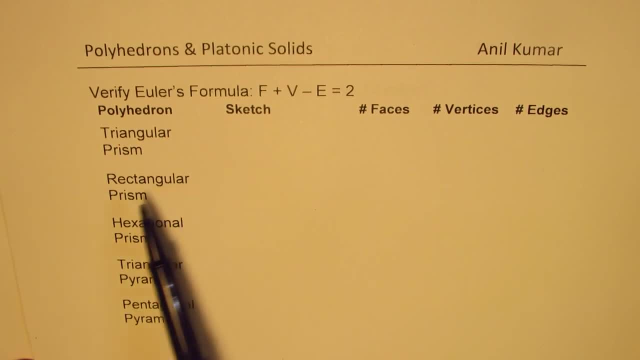 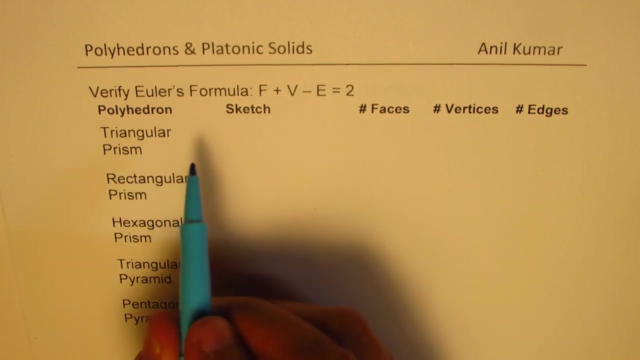 here. So we will talk about triangular prism, rectangular prism, hexagonal prism and then triangular pyramid, pentagonal pyramid. So let us sketch these and then we will count how many faces, vertices and edges they have. Triangular prism means we have a triangle. 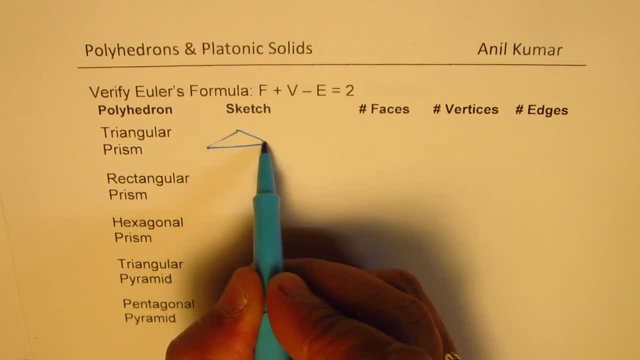 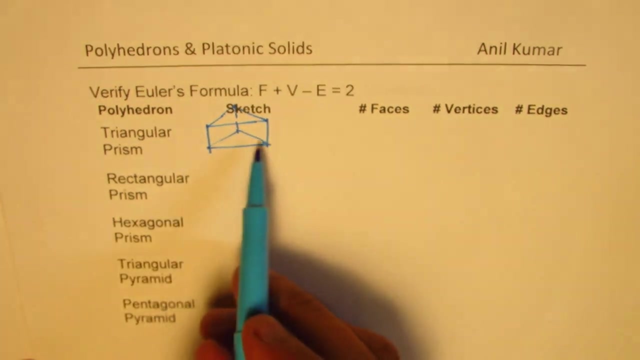 here let's say: right, and prism means exactly similar triangle on the top also, right? So let me just okay, And then you just combine, join them together, Okay, And then these edges, right. So the shape which you are seeing is called triangular. 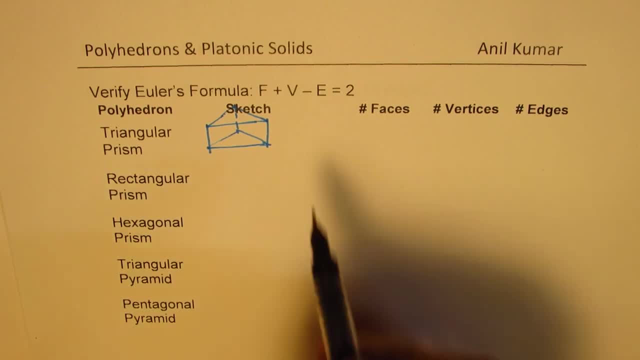 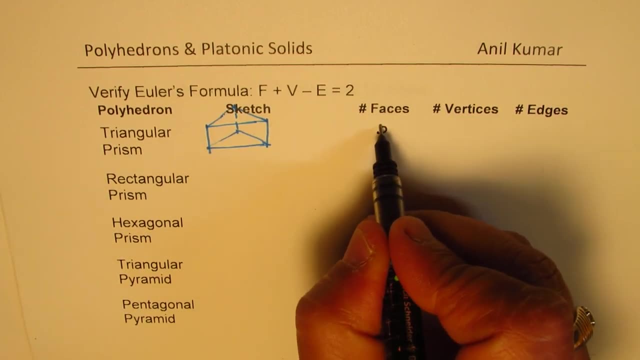 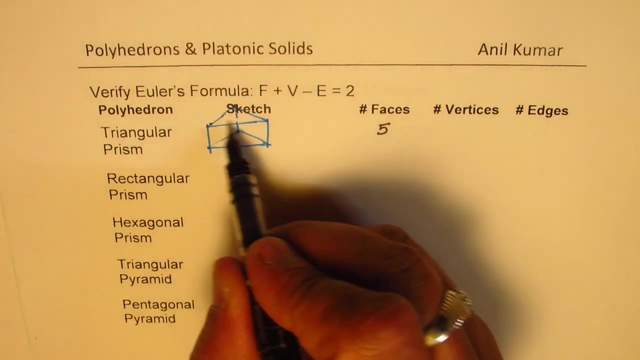 prism right Now in this shape. how many faces are there Top and bottom right And then these three triangles right? So we have five faces here: top and bottom, two and three. on the sides. Vertices are one, two, three, four, five, six And the edges three and 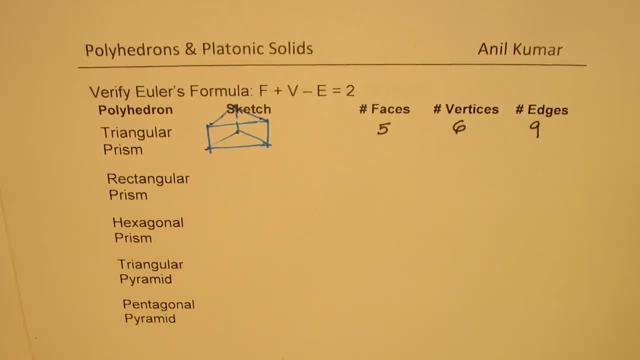 three six And three nine. Do you see that? So that is what we get Now, if you check face plus vertex is how much? Five plus six is eleven, and eleven take away nine is two, right, Do you understand? So the formula works here, right? Similarly, what you can do now is just: 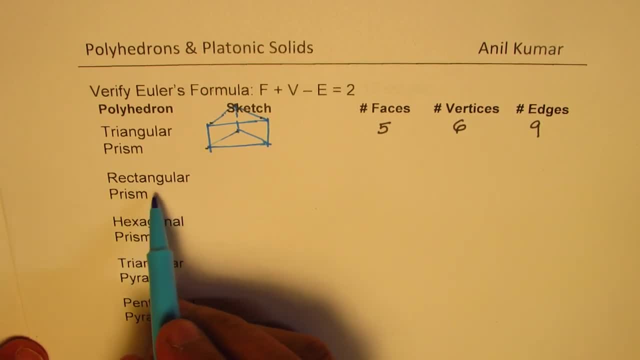 pause the video and fill up this table. So we have a rectangular prism. So last time I made a pyramid, Now we will make a prism. So make a rectangle right here. This is the here, like this, and whenever you're making a prism, just make exactly similar. uh, on the top, correct? 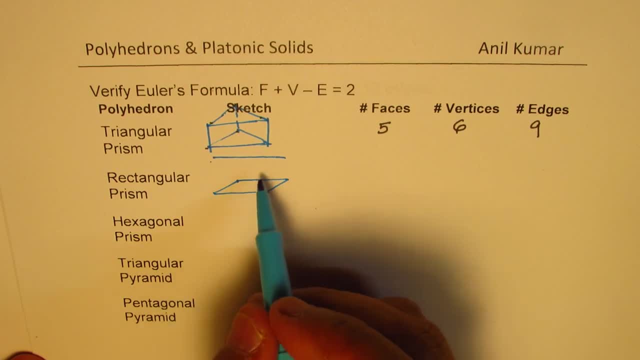 so. so we have kind of like this right so. so that is the base. anyway, i went slightly, i should use different color, okay. so we'll use a different color and then squeeze it in, okay. so let me just uh say that this is, let me just redo it right. so i'm making it shorter, since otherwise it'll mix. 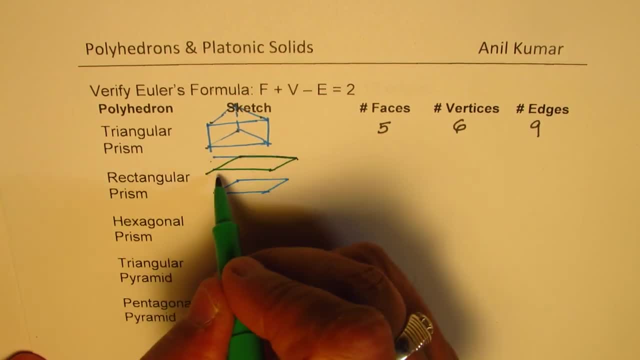 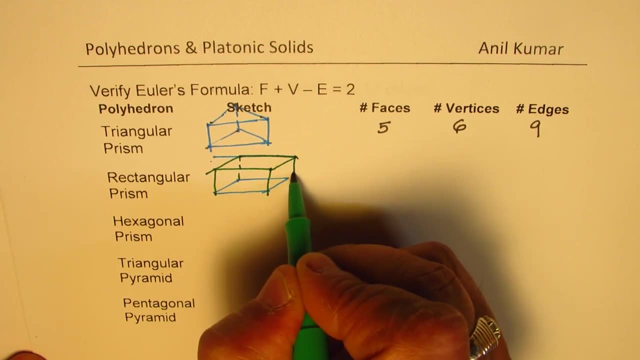 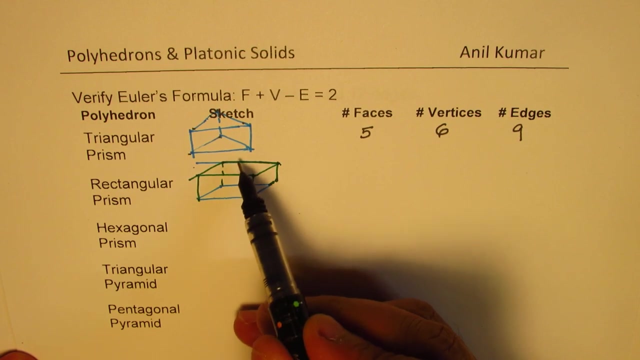 that up. right, so we have this one. okay, so that is our top. and then when we combine: uh, these, you see, right, this is slightly wrong, anyway, you good, now let's count the faces: top and bottom, that is two, and four on the sides, so we have six faces. what is this? 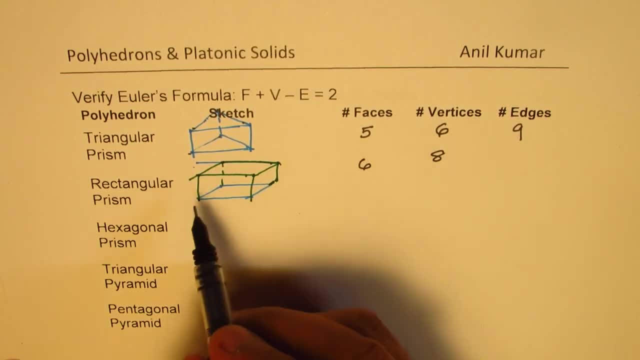 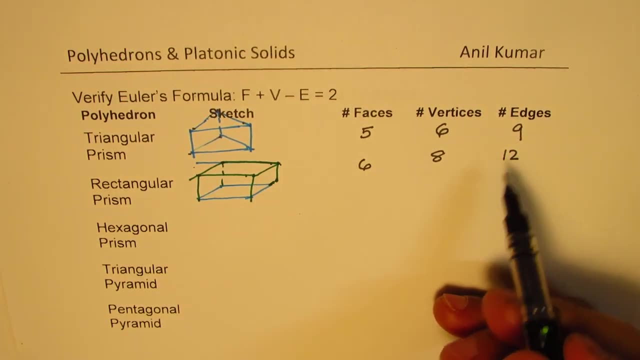 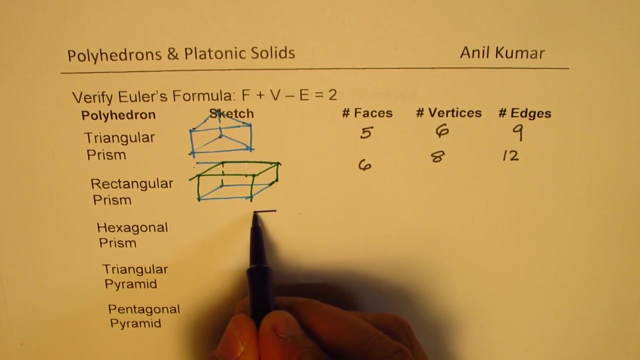 one, two, three, four and four. eight edges: four, four, eight and four, twelve. now again, if you do your math, which is: adding these two is fourteen, right, and take away twelve is two, so it works right. hexagonal prism means that you have two hexagons now right, so prism means we have two hexagons. let's just make two hexagons, right. 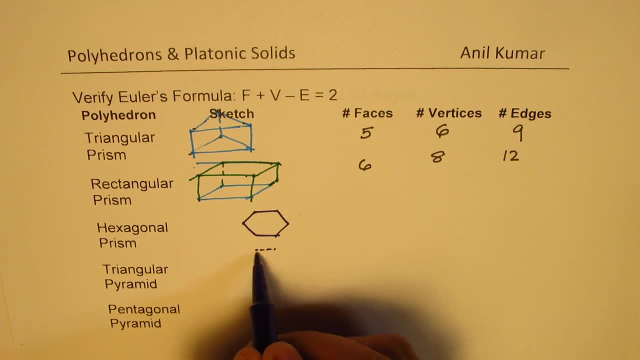 one on the top and then we'll make uh one at the bottom, correct? so this is uh the side which is on the other side, and we'll just make this and join these points. right, so you can join these points which are the vertices. it makes sense, right, slightly better than before. 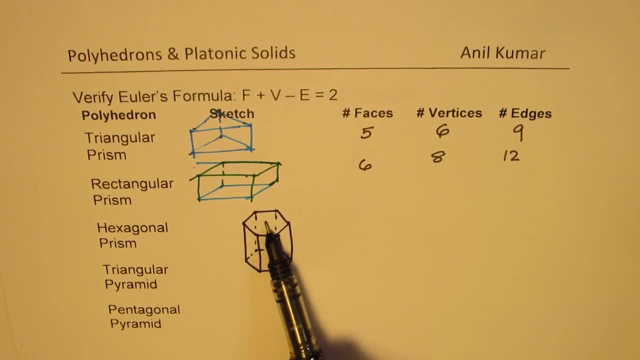 hexagonal, will have how many faces? hexagonal faces on top and bottom, two hexagonal faces and six of these which are rectangular right. so we have eight faces. what is this? six on the top, six in the bottom, which makes it twelve edges. six on the top, six in the bottom, twelve and those standing? 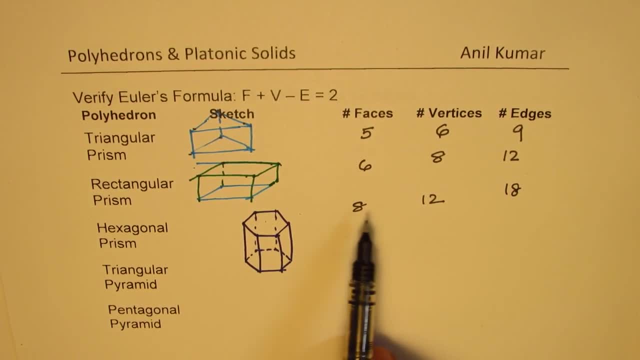 vertical is six again, so it is eighteen. when you add eight and twelve you get twenty, and twenty minus eighteen is two. so it works. you get the idea right now we're talking about the top and bottom, so we're talking about triangular pyramid. so that was a prism, so let me again sketch a pyramid here. 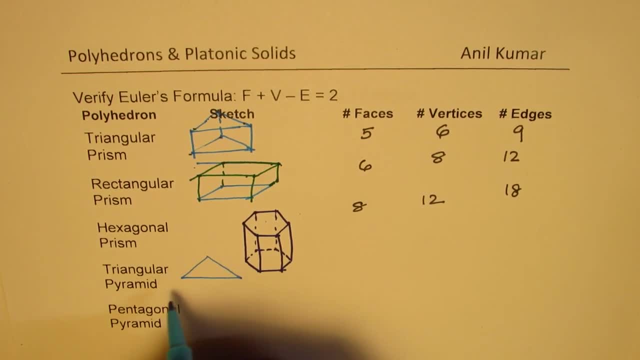 so we have now a triangle here, right, something like this, and pyramid means we'll just connect it with one point on the top. that's what you get now. in this case, number of faces is one triangle in the base, three on the side, all triangles, four in all. correct as far as the vertices are concerned. 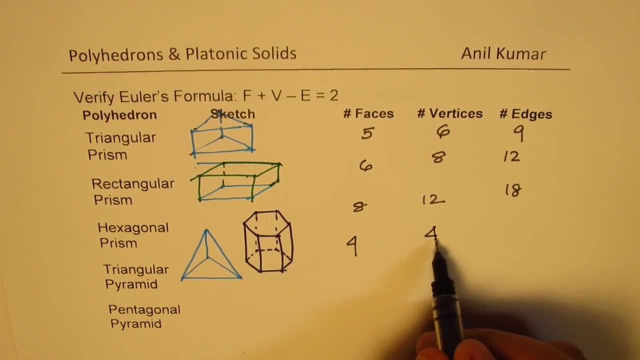 so that's the first point. so we have two sides, one two, three and one four. four plus four is eight. we are expecting how many edges? six, that is true, three in the bottom and three standing. so it works. do you see that? now the last one here is pentagonal pyramid, right, so we have to sketch pentagon. 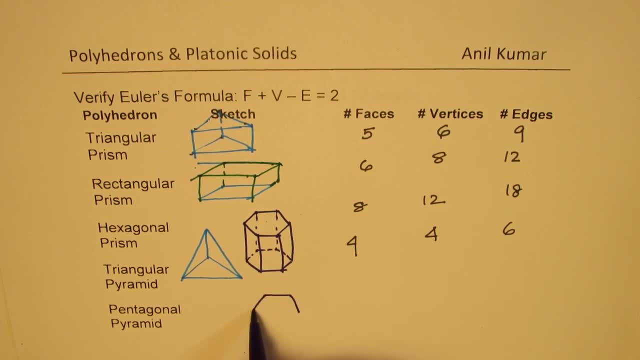 so pentagon will have five sides, so we have one. so let's say two, three, five sides, and pyramid means there'll be only one point on the top and that gets connected with all of them, right? so so let me just take one like this, so that you know we could actually show you. 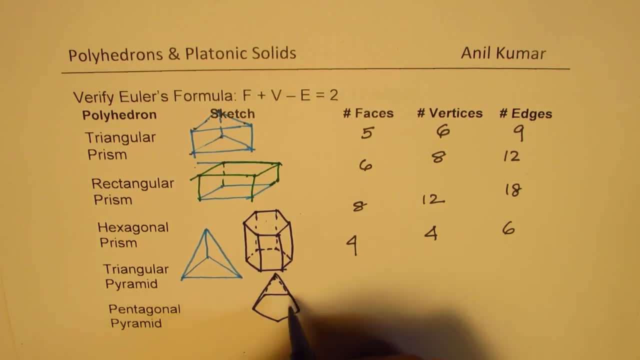 uh, how it looks like. is it okay? all right, so something like this: so that is your pentagonal pyramid. which has how many faces? one at the bottom, which is pentagon, and then we have all these triangles. so whenever you have a pyramid, we have triangular faces right, five of them, five. 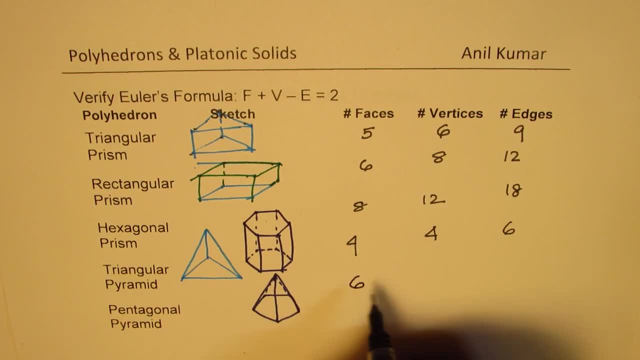 plus one is six. so we have six faces in all. as far as the vertices are concerned, five plus one, six, that makes us twelve. we expect ten edges, right, five and five, ten. that makes sense, correct. in each case, you will find that the number of faces plus number of vertices, minus the edges, is 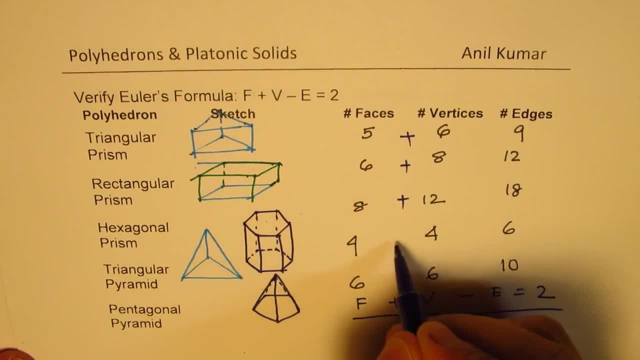 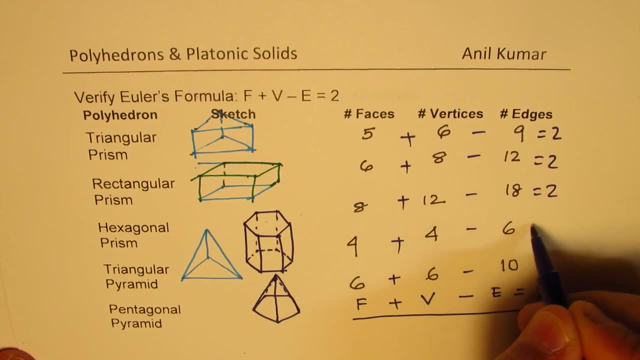 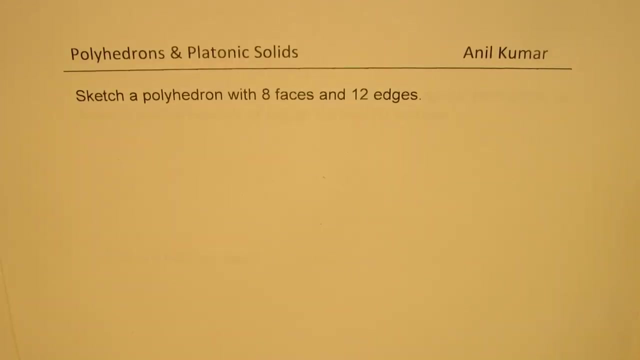 so i like you to calculate right these values right and then see if you really get two for each right. if you do, then the formula works. otherwise you've done a mistake. right formula always works for a polyhedron. okay, now we'll talk about sketching a polyhedron with. 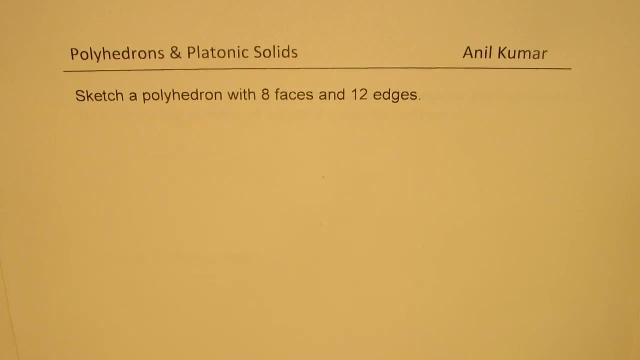 eight faces and twelve edges. how can we do that? okay, so important thing here is to figure out how many vertices right? so let's get back to this formula: phase plus vertex minus edge is two, right, so we have the formula which is: phase plus vertex minus edge equals to two. we are saying: 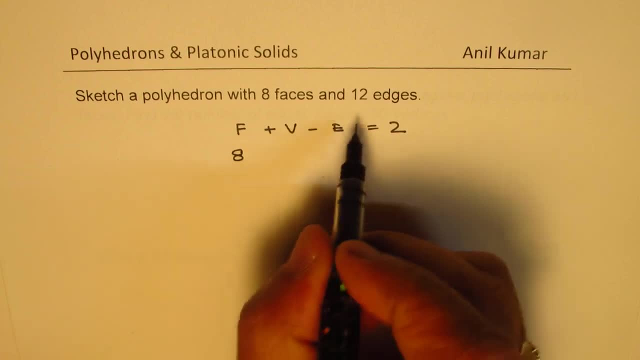 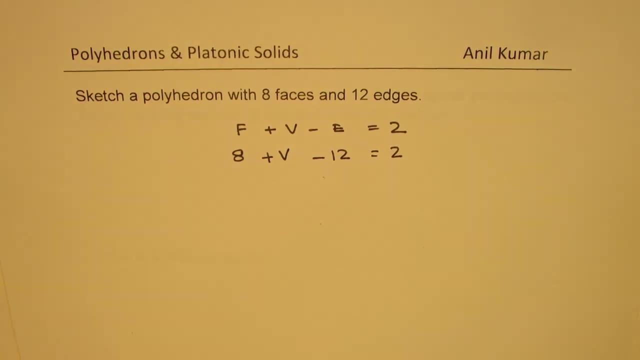 to sketch a polyhedron with eight faces, right. so eight and twelve edges minus twelve, which is two. so we need to find how many vertices are there, correct? so let's figure this out. so what number will give me two here? so that should be how much. that should be actually, uh, seven or six. what total has to be fourteen, right? 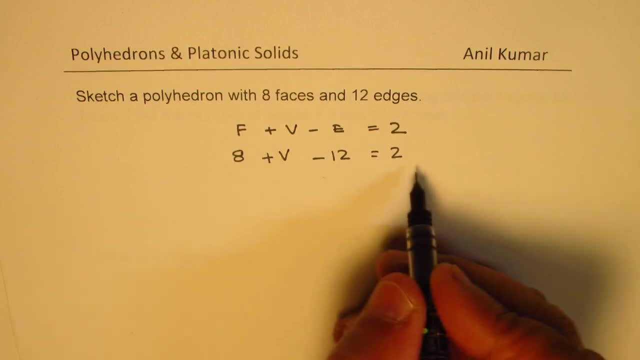 so we expect v to be six. or you could calculate like this: v equals two, two point eight. so when we talk about sketching a polyhedron with eight faces, let's get back to this formula. so what number you take is seven and twelve. take discount two. take this twelve on this side, take away eight, is that. 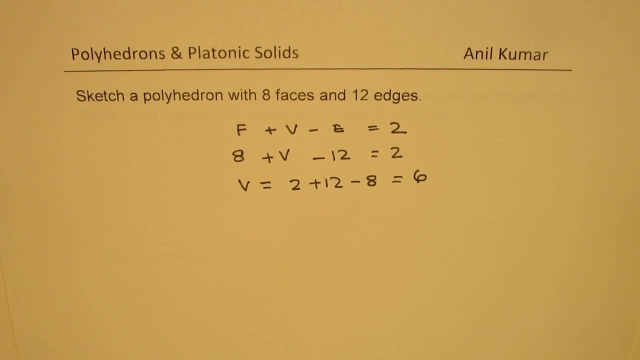 correct. so we have fourteen, and from fourteen you take away eight, which gives you six either way. so we have six vertices. now, with six vertices, you have to sketch a polyhedron. the solution is something like this: well, we have six vertices, so one is, let's say: these are my four. 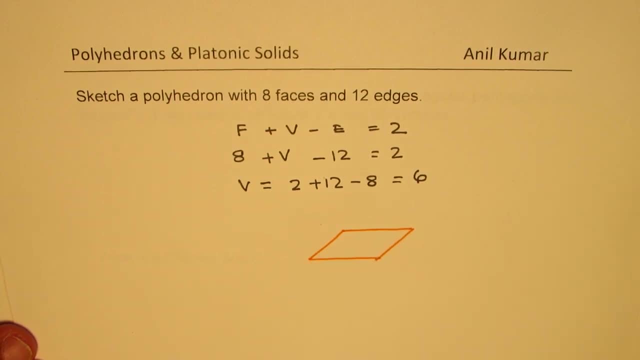 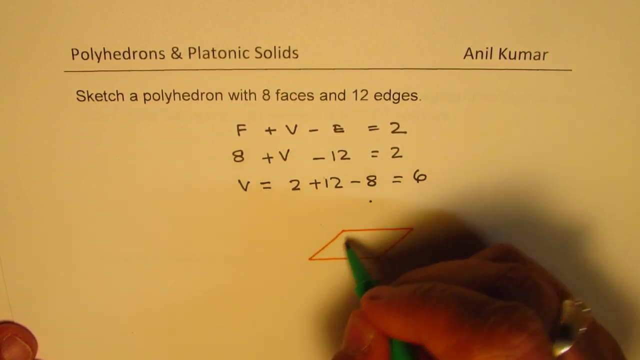 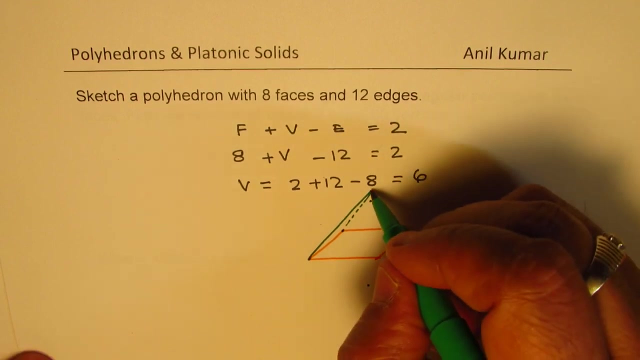 which i'm doing like this, and then we have one on the top and one at the bottom. so what happens really is that we can just combine, let's say, let's say this one like this, right? so? so i purposely shifted it a bit so that you know, i could clearly show you a drawing. 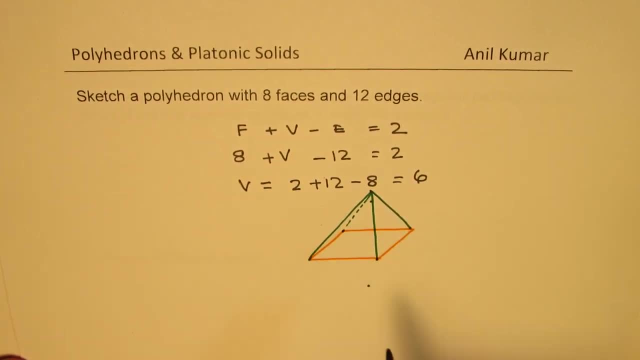 so that becomes the top right. so we have, you see that, and this is the bottom part. so something like this, correct, so that shape has got eight faces. you can see one common right and then four up, correct, and we have four down right. so each so outside, if you're looking at, don't count. 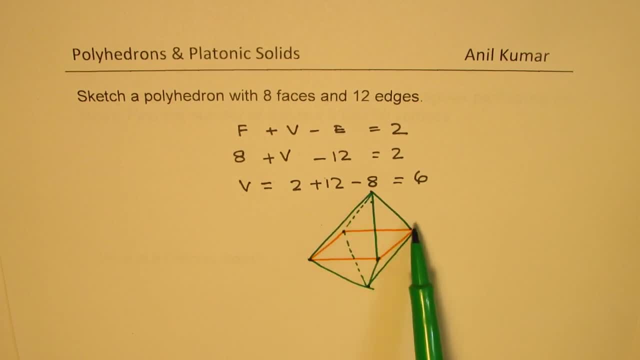 this thing in between, only these triangular faces, right? so what we have here is we have eight triangular faces. okay, don't count this. these, these are getting joined. okay, and it is not a face. think it is hollow from here, is it okay? so that is not a face. however, it does combine with your edges. i mean, i should have drawn a. 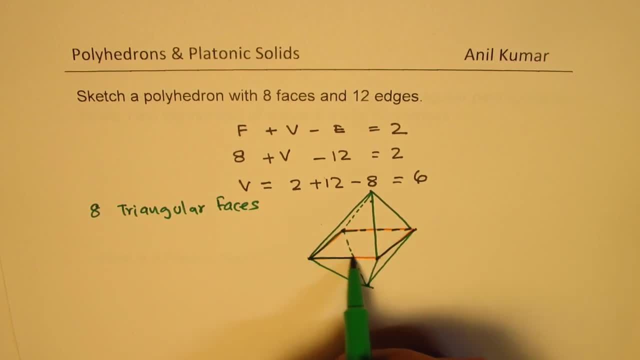 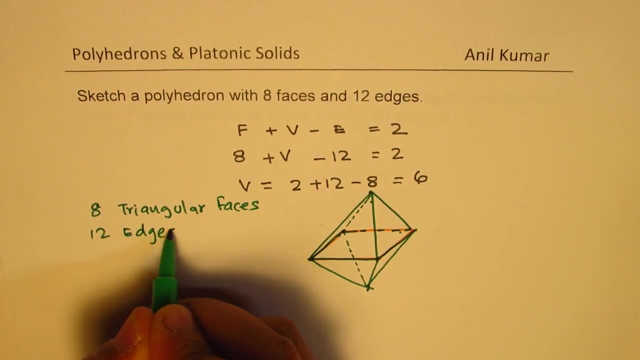 dotted line correct. so that is how it is. the number of vertices are clearly one, two, three, four, five and one six. okay, six vertices and the edges. so as far as the edges are concerned, we have four on the top right Now. we will learn more about this diagram soon. 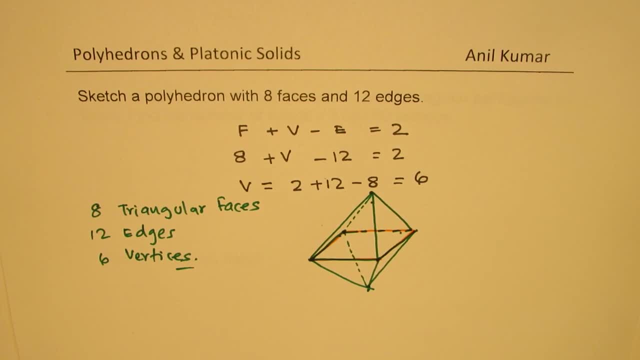 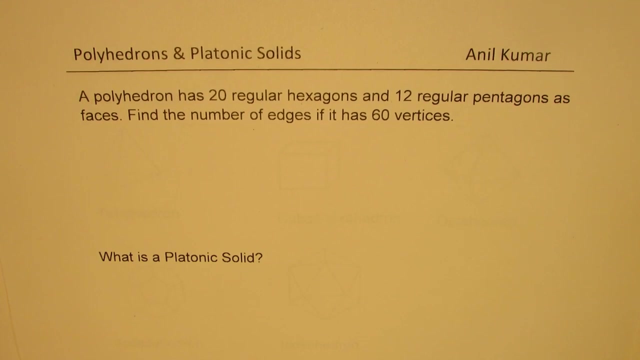 right, but for now that is the shape, which is a polyhedron with eight faces and 12 edges. okay, now next question. here are two other questions for you question is: a polyhedron has 20 regular hexagons and 12 regular pentagons as faces. 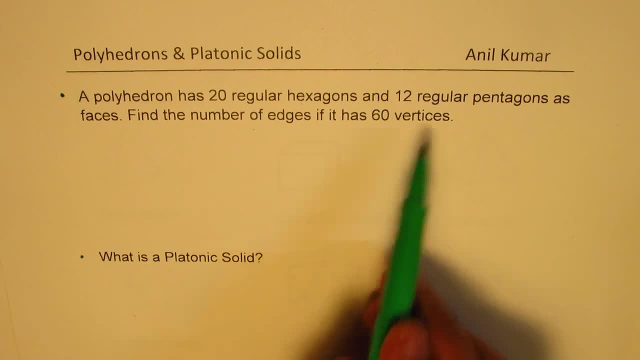 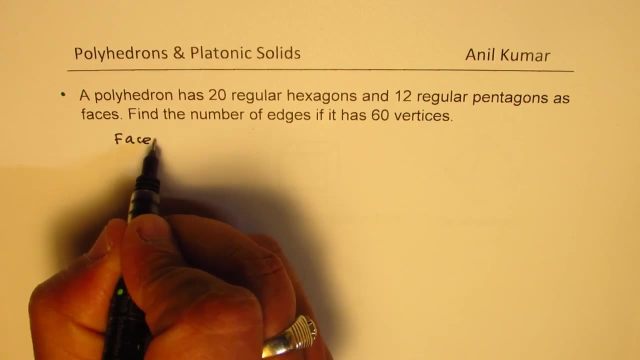 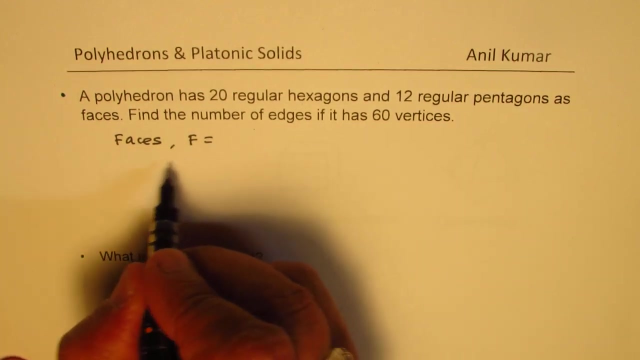 find the number of edges if it has 60 vertices, right? so i like you to pause the video and answer this question. so it has some faces. which is given to you, right? so f is given to you, and number of edges: find the number of edges. we don't know vertices. we are given, so we know vertices. 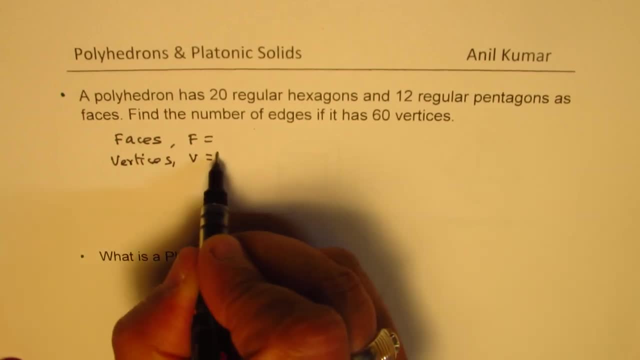 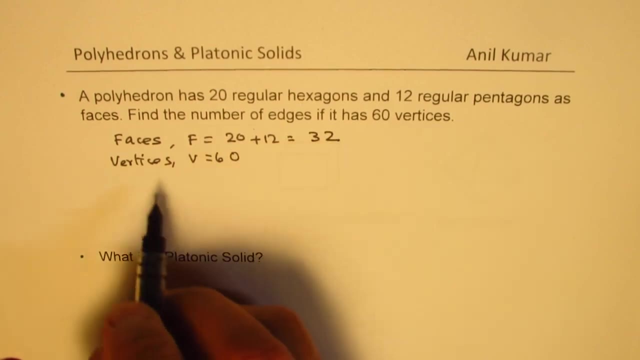 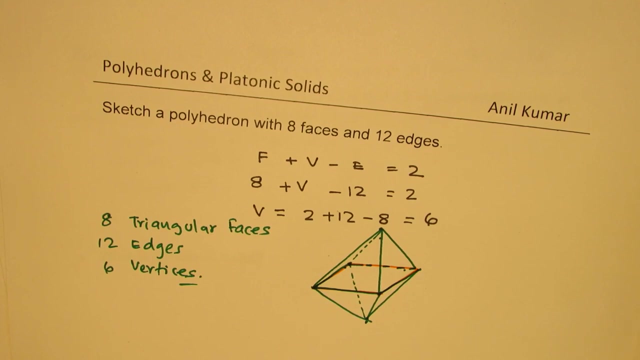 is v is 60, for us, faces is 20 plus 12, do you see that, which is 32, and we need to find the edges e. so how will you find edges? well, again, use the same formula, right? so that's a very important formula. edges are maximum, remember that. so faces plus vertices, the formula here again is: 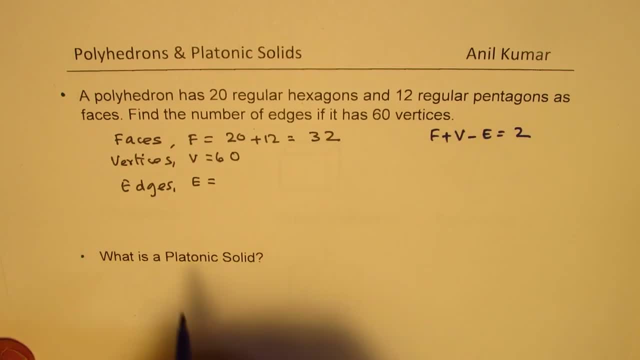 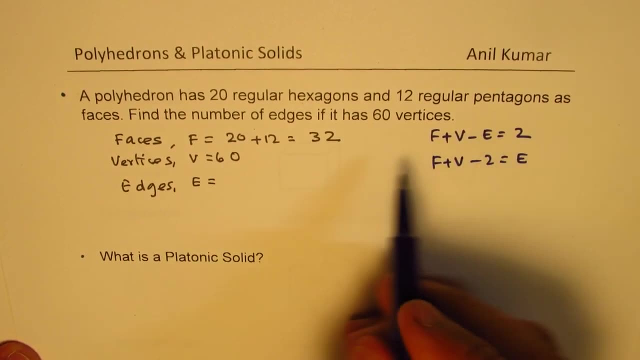 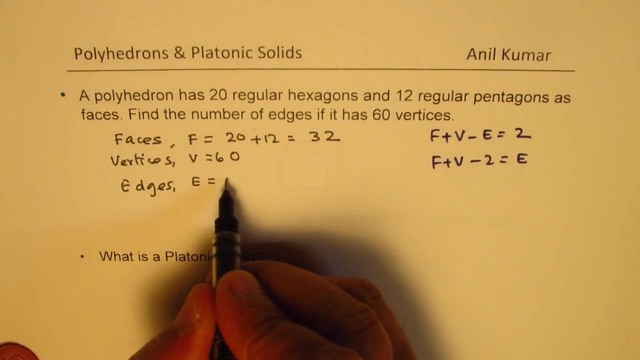 faces plus vertices minus edges equals to two. we want to find edges so we can say faces plus vertices minus two is edges correct. so you can add these two and take away two. that should give you the answer right. so let's do it. so: faces is 32 plus 60 minus two, so that 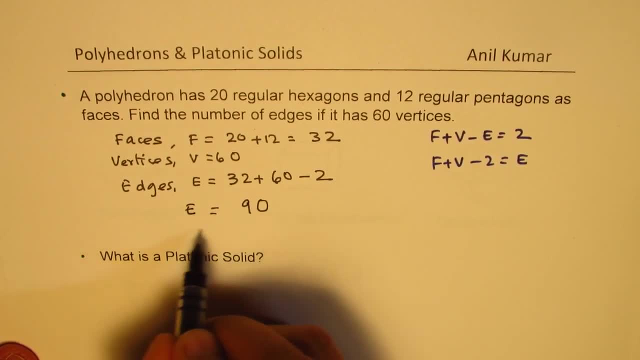 gives you 30 plus 60 as 90 edges, do you get it? so the number of edges is 90 for this particular case. perfect. so that is how we are going to answer this particular question. now here is another very interesting question, and that is about platonic solids. what is a platonic solid? now, that's a very 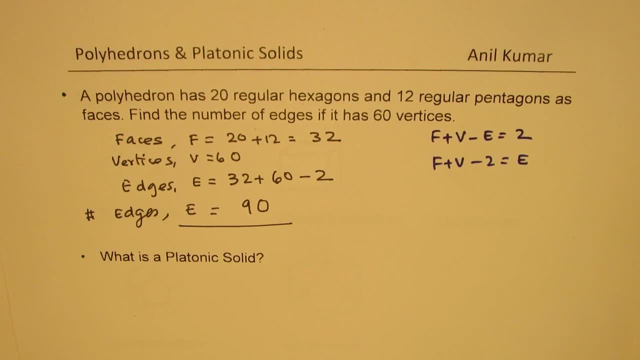 common term most of the time used whenever we talk about polyhedrons, right, so? so in a polyhedron, there is a special kind of a polyhedron. where we have this is a special polyhedron, so what is special about it? one we have a regular polygons. 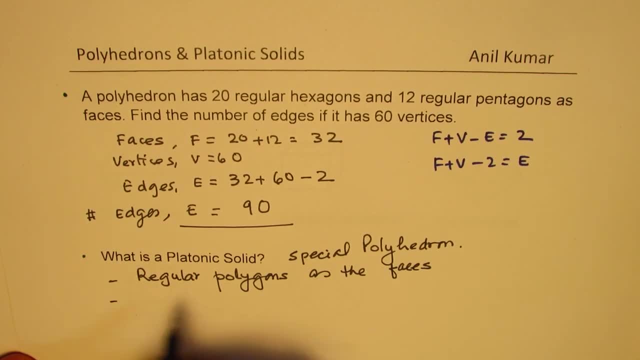 as the faces. okay. regular means all polygens like, all sides equal, all angles equal, okay, regular polygons has faces and all angles equal. so regardless of the determining positive stuff at all methods, the of the does not mean Box. he and his product are equal. the opposite, he cannot be combined. so many points looking in this: Pauli sugar: Polyhedral, polyhedron, polyhedron, polyhedron surrounding the polyhedronheadr means polyhedron, rich polyhedron, polyhedron're scared at the baptism earlier. you'll know the. 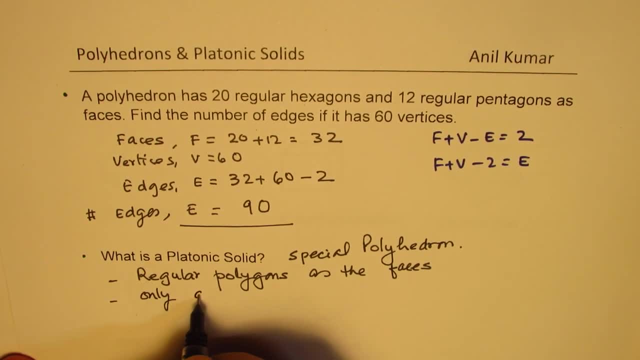 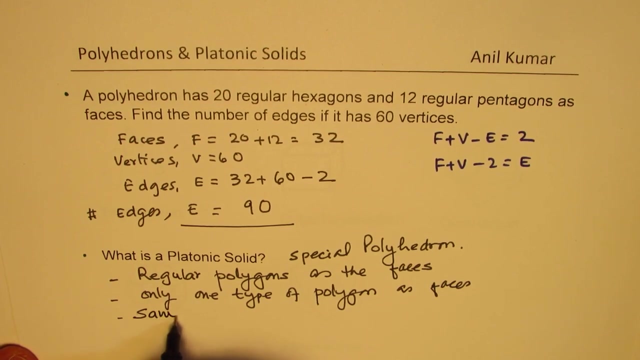 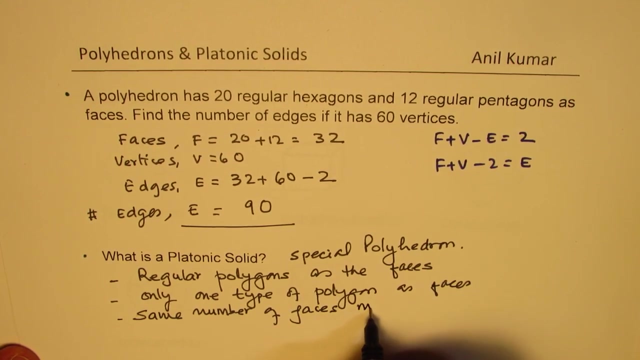 Polygons as faces and only one type of polygon, not combination of two as you saw in pyramids. You see that. So that is kind of very important to understand, right? So that is important. So same number of faces meet at all the vertices. that is also important, correct? 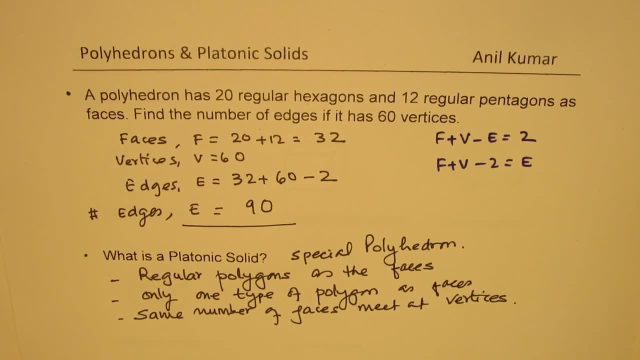 So these are distinguishing features of a platonic solid. right. So a platonic solid will always have regular polygons, All the polygons as its faces, all the polygons will be of the same kind, right? So if we have triangular, all will be triangular. 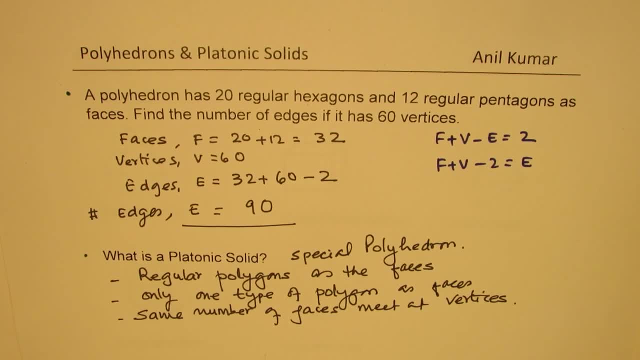 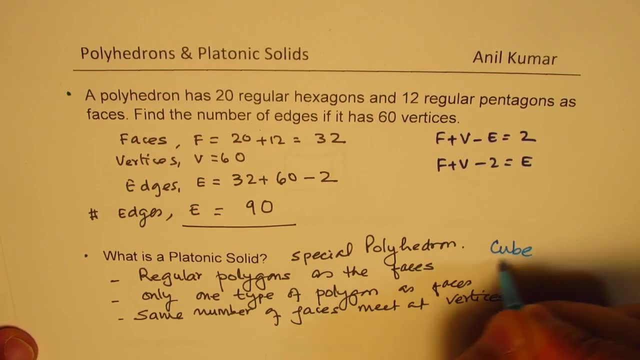 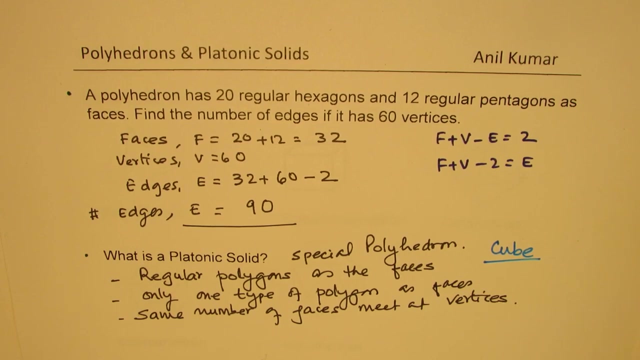 If we have pentagonal, all will be pentagonal. That's what it is right. If we have square, like a cube, right Cube is a good example. So cube, all are exactly similar polygons, squares, right And all of them they meet at same number. 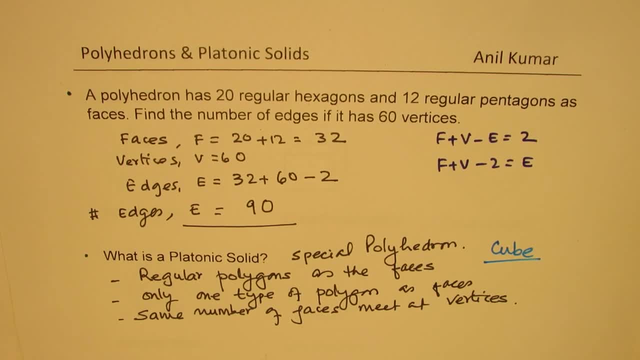 So then, these three, what are the three kinds of polygons? The first one, the most common one, is tetrahedron, And the second one, the most common one, is tetrahedron, And these are the five kinds of polygons that we have here. 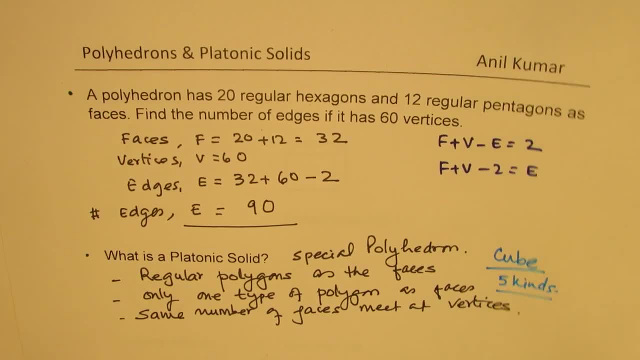 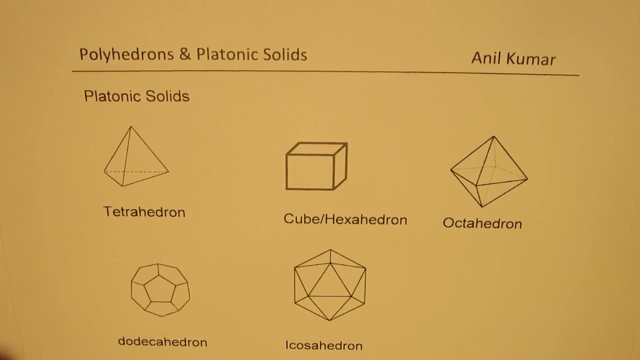 You know what are these five kinds? Let's have a look at these. So the next page gives you the figure of these five kinds of platonic solids with their names. So the most basic is tetrahedron. You see all triangular faces in a tetrahedron, right. 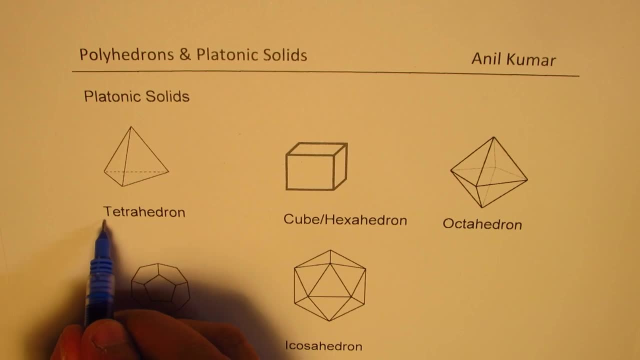 So we see 4, tetra means 4, this thing, tetra means 4, 4 tetrahedron, right. So the polygons, the number of polygons here are 4, right. So what we see here is that there are 4 faces. 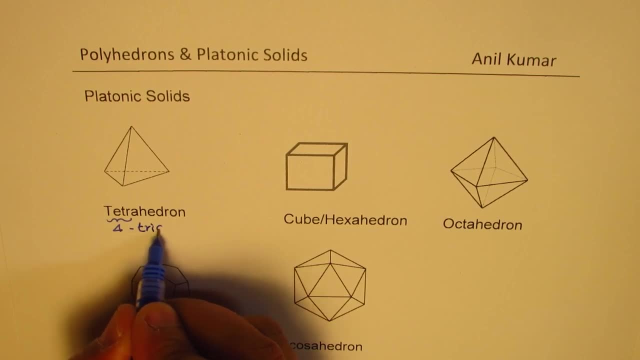 So we have 4 triangular faces, correct? So that is kind of very important to understand Now at each vertex how many faces intersect. So let's look at this particular vertex, for example. So at this vertex 3 faces intersect, right? 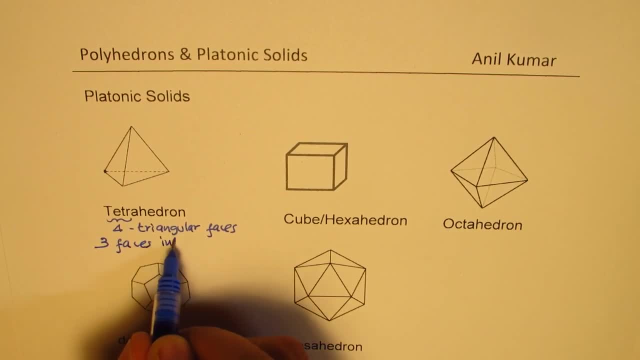 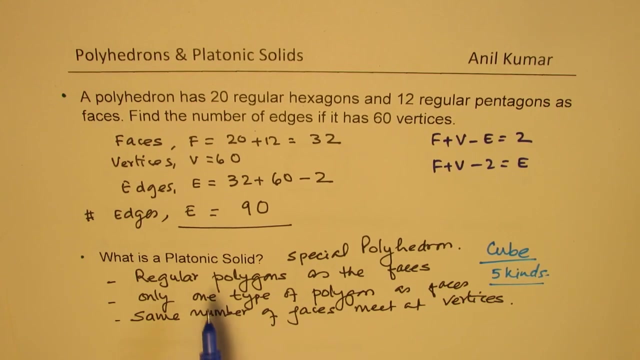 So 3 faces intersect at each vertex. So, as we pointed out, for a platonic solid it is very important that all have same polygons, regular polygons, right And only one type of polygon, and same number of faces meet at each vertex. 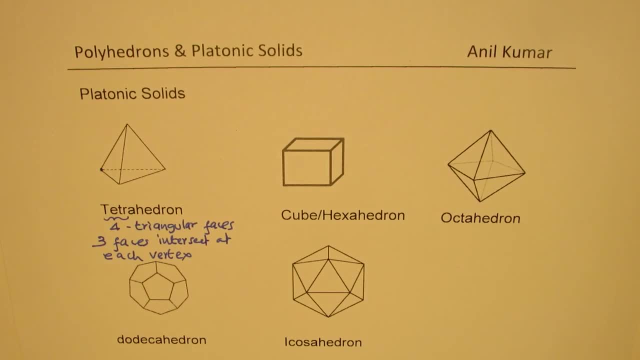 That is important, right? So what we note here is that there are 3 triangles which will meet at each vertex. Each vertex, there are 3 triangles, correct? So that is a tetrahedron. Now, cube is also called hexahedron. 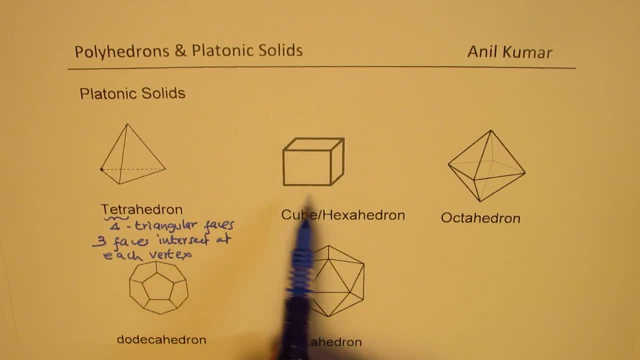 Hexahedron, since it has 6 faces right. Hexa means 6, right, So this means 6 faces. So we have 6 square. so that means a regular figure, right, 6 square. and these are triangles, and these triangles are equilateral triangles. okay, 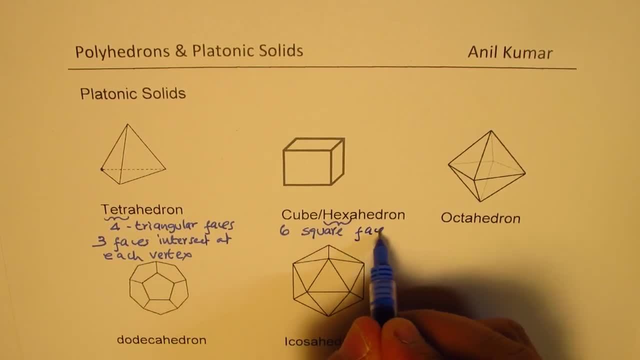 6. Square faces. So at each point, as you can see from here, you will note that let's take this point right. So 1,, 2, and 3 faces meet at each point, correct 3 faces intersect. 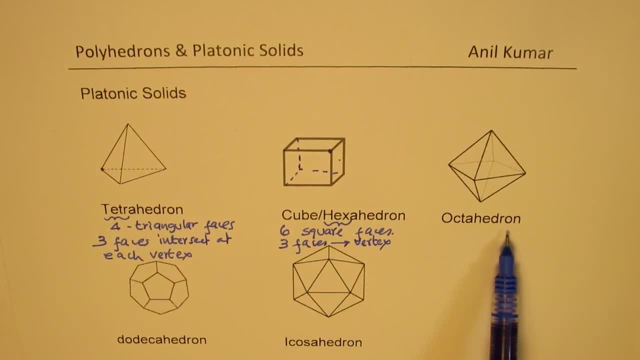 Clear. Octahedron is something which we just drew right, So what we had sketched earlier was actually octahedron. So I hope now you understand the properties of this octahedron. It has triangular faces, right. 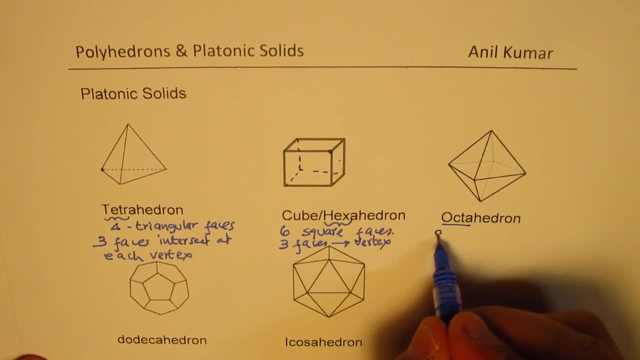 So octahedron has, as the name suggests, 8 triangular faces right Now, at each face, at each vertex, let's say this vertex. So how many triangles are meeting at this vertex? 1,, 2,, 3, and 4.. 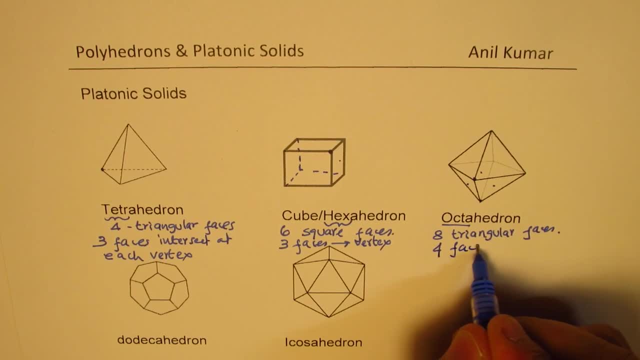 So we have 4 faces meet at each vertex. Is that clear to you, right? So at each vertex there are 4 faces which are meeting, right? So here, if you consider this one, we have 1,, 2,, 3, and 4, right? 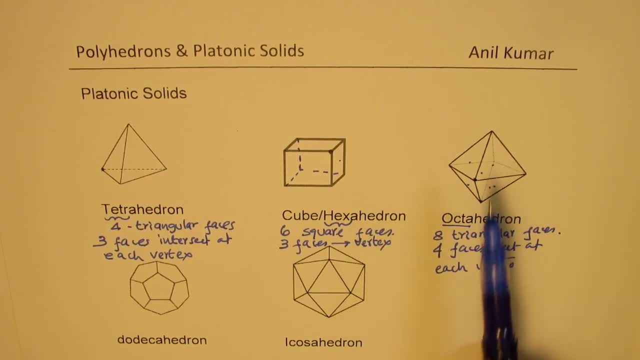 So 4 faces meet at each vertex and the name is octahedron. The next one, as you can see, here we have pentagonal faces, So we have actually, in this particular case, we have 12 pentagonal faces.